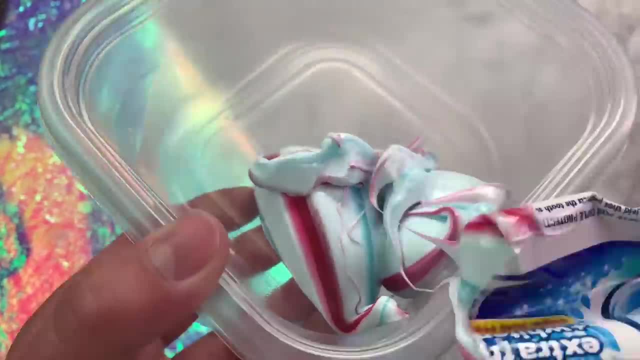 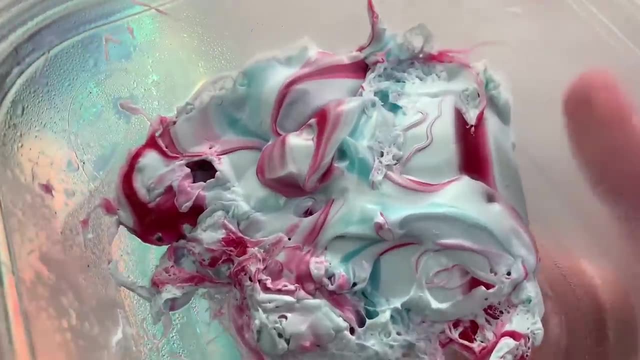 I have my toothpaste in my container, so now I'm just going to microwave it. I took my slime out of the microwave and, as you guys can see, it looks pretty sticky, so I'm just going to mix it to see if it turned into slime. 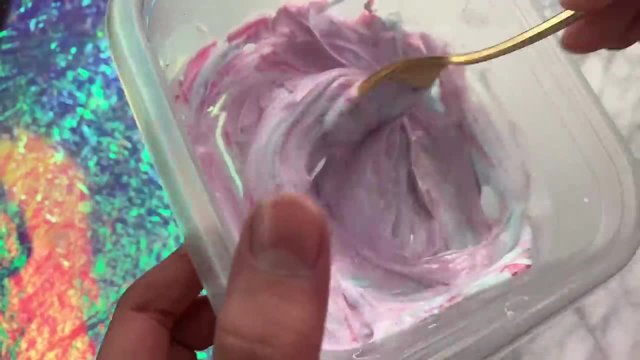 As you guys can see, unfortunately the slime recipe didn't work, but if you guys have any other toothpaste slime recipes, be sure to check them out. I'm going to be using this one right now. I'm going to leave them in the comments below. 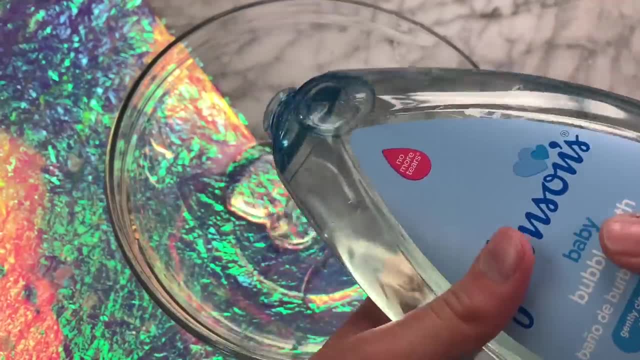 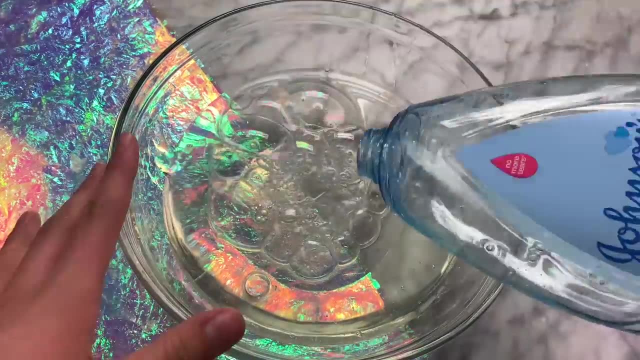 I'm going to be showing you guys a new way to make clear jiggly slime. You're going to be needing some Johnson shampoo or any sort of a jiggly clear shampoo. You just want to add a container of that into your bowl, or add a half container and then 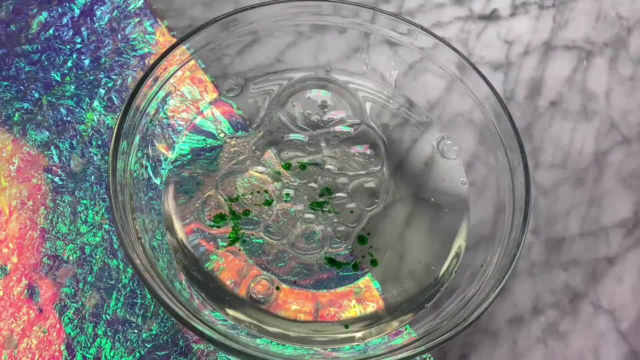 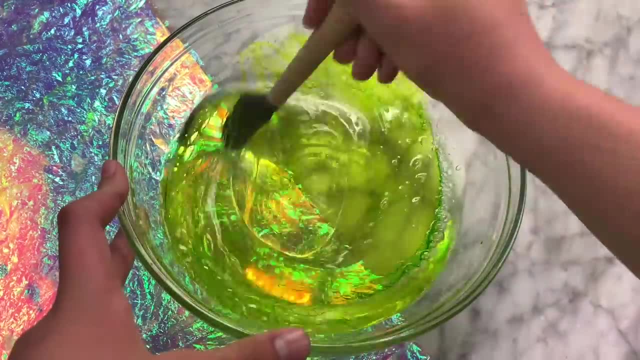 you want to dye it to whatever color you want it to be. I'm just going to make mine a bright green color and I'm just going to mix all of my food coloring in To make our slime super jiggly. you're going to be needing some water. 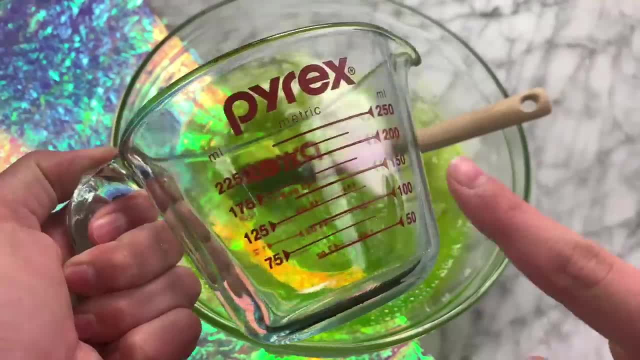 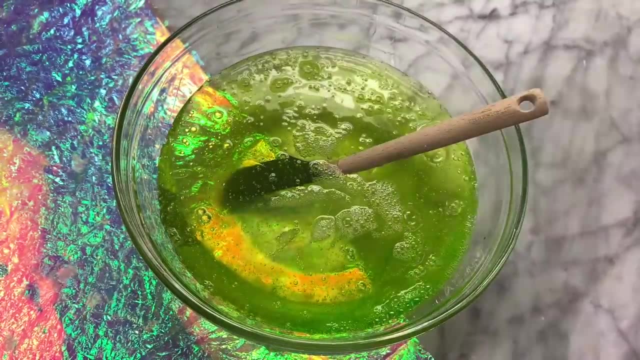 So the first thing we're going to be doing is adding in water. I'm planning on adding 400 milligrams of water, and I already have 500 milligrams of soap in my bowl, so I'm going to start off by just adding in the 250 milligrams, and then I'm 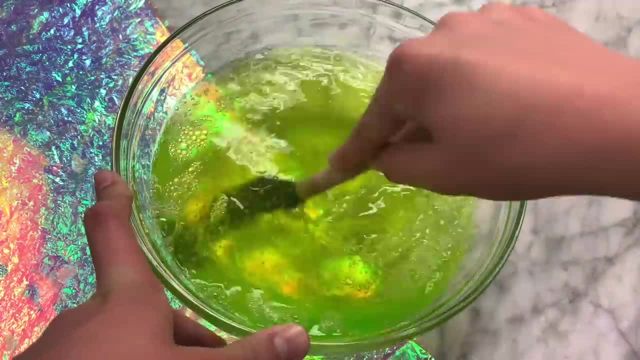 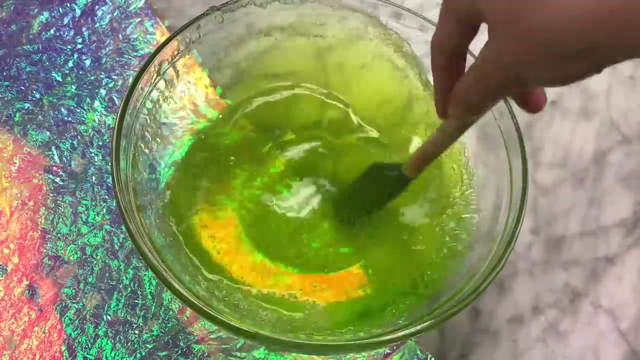 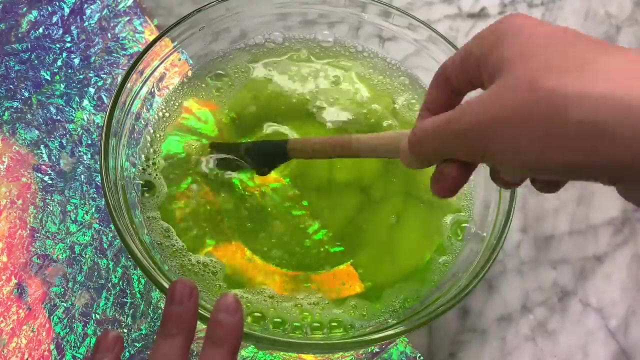 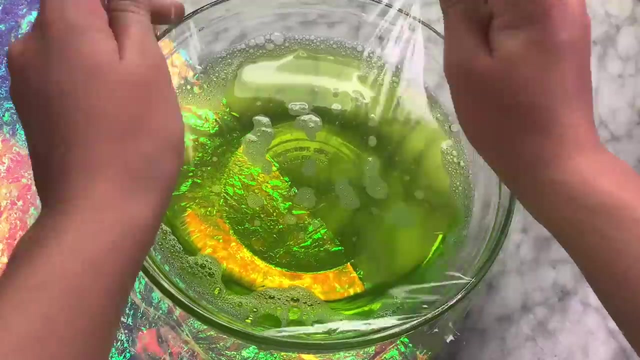 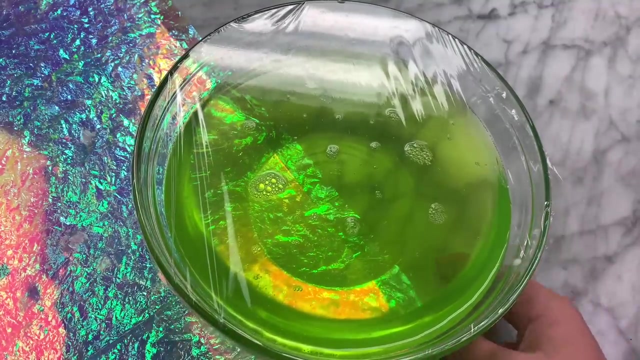 going to add in some more once I've mixed this all up. This slime has a consistent texture. it is time to let it sit, and for this we're going to be drying it out by putting in some surround wrap on the top of it and then just letting. 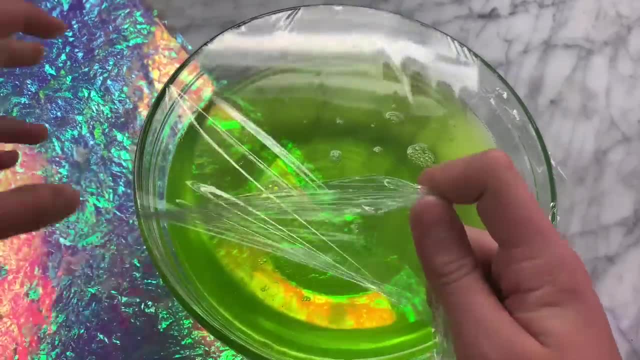 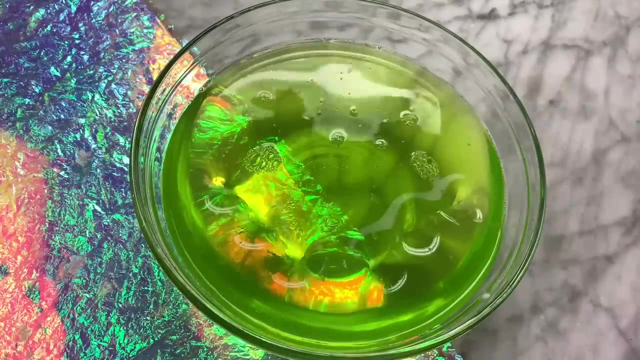 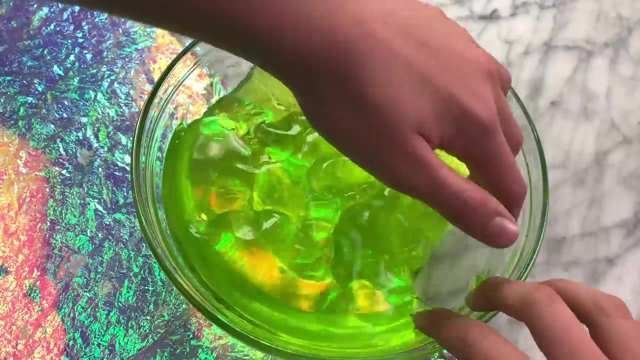 it sit for a couple of days. Mine took two days to sit, but yours might take longer. so if yours is still looking watery, just keep letting it sit. Once I've left it in the fridge for a couple days, I'm just going to pour this onto the 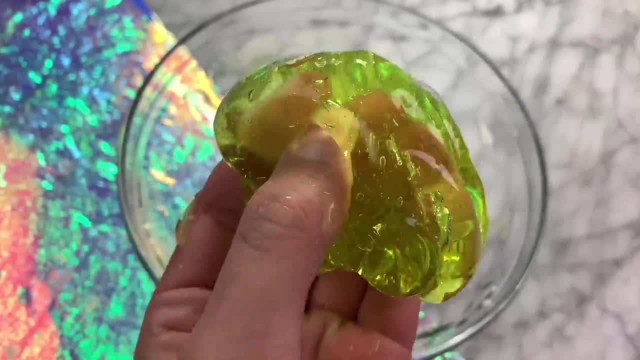 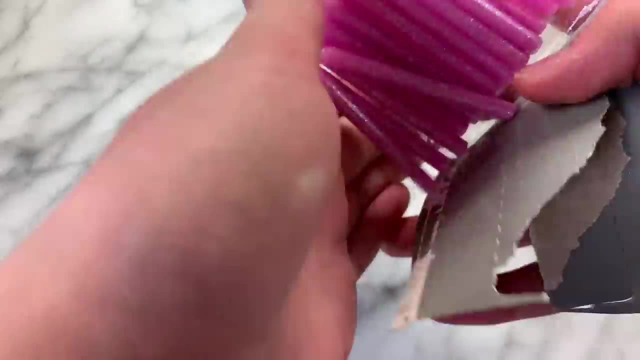 bowl and then I'm just going to shake it. so the�� So with the no glue slime recipe. I will be trying out the brand new birthday candle: no glue slime recipe. drawings for the recipe. basically, they just melt candles and they add a face mask to them. 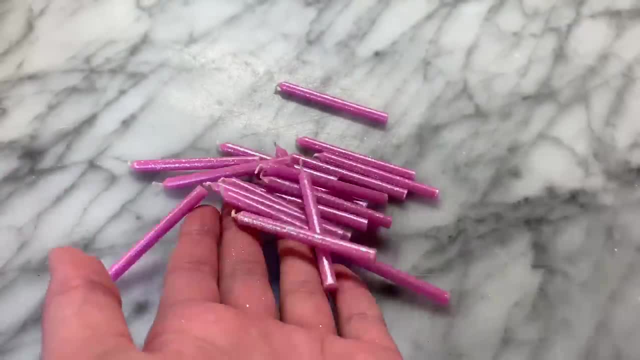 and it makes a perfect slime. Last October's water slime video: I did make slime out of a candle, so hopefully this will work too. I just microwaved a bunch of the candles and they're not melting, so I'm going to take a. 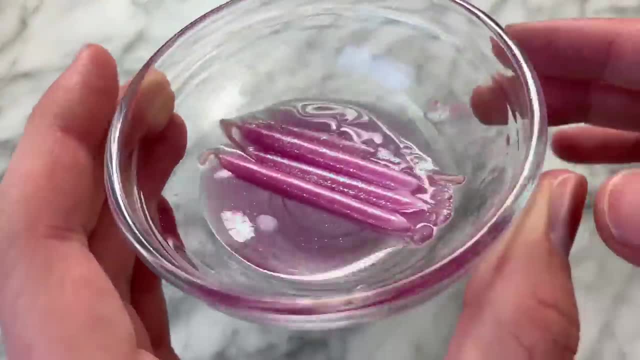 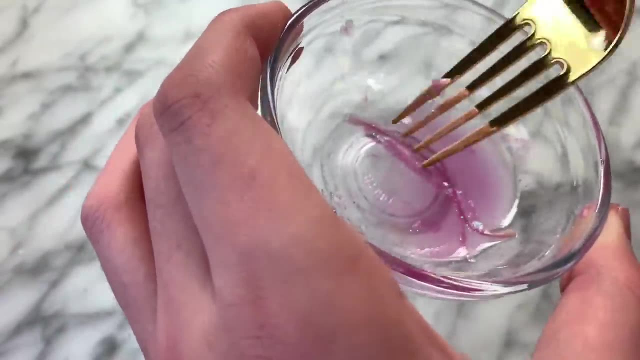 few out will help it melt a little bit better, so i'm going to pop these ones in the microwave too. here are as much as i could get of the candles to melt, so i'm just going to take the rest of the candles out and we're going to try to add the face mask into this little bit of melted wax. 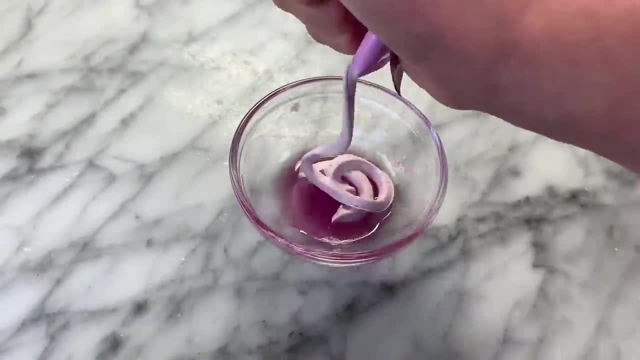 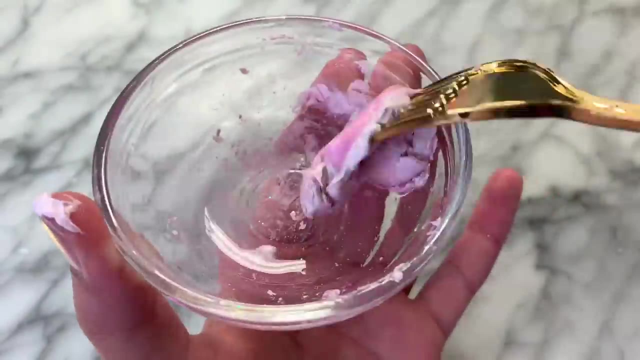 i know goose iron recipes usually have peel off masks, except for this. one's just a mud mask and that's what they used in the video, so i picked this one up that i had actually lying around in my house. i was hoping the candle wax would start drying again and basically face mask a harder. 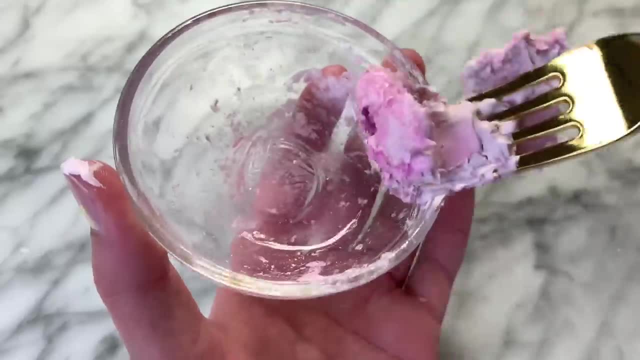 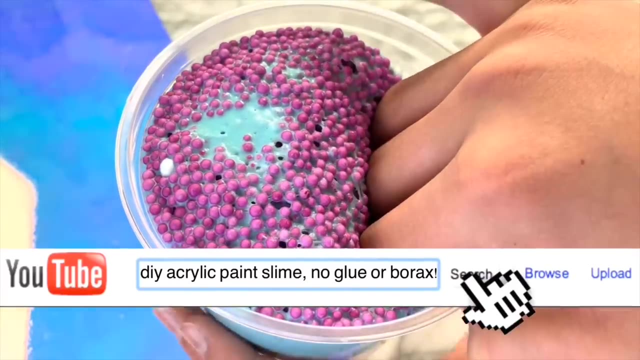 consistency. so it would be like slime except for this didn't work and it basically just left us with the same mud mask we had before. so this recipe was a fail. the next no glue slime recipe i will be showing you guys how to make is no glue acrylic paint slime you most likely already will. 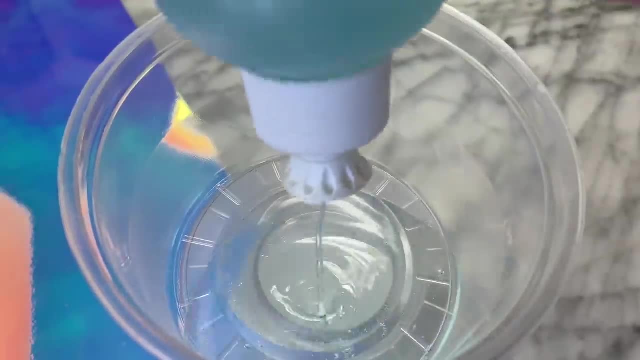 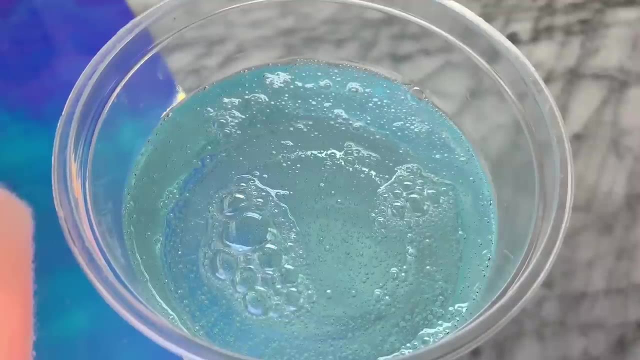 have all the ingredients to make this slime, so let's get started. first ingredient you will be needing for this slime recipe is dish soap. i got this one from target. it was only 40 cents. you need about a cup of dish soap, and then you're also going to be doing some shampoo. 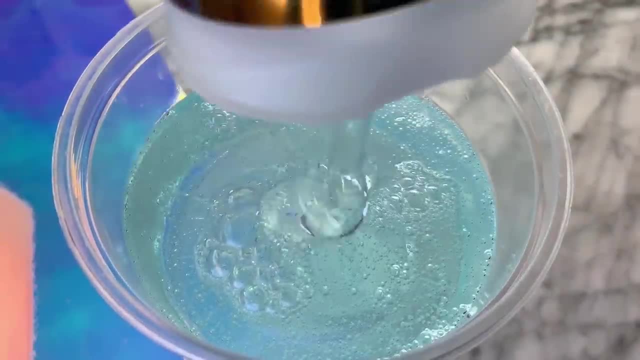 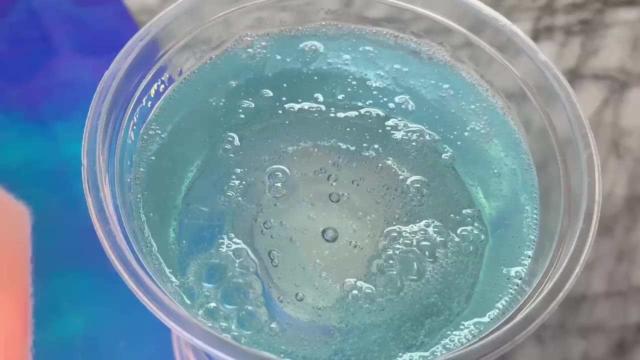 and for shampoo. you're only going to be needing to add a tablespoon of shampoo into the dish soap, so i'm going to be using this one, and i'm going to be using this one to make a slime. next ingredient is pretty crucial to this recipe, and that is acrylic paint. so i have this acrylic. 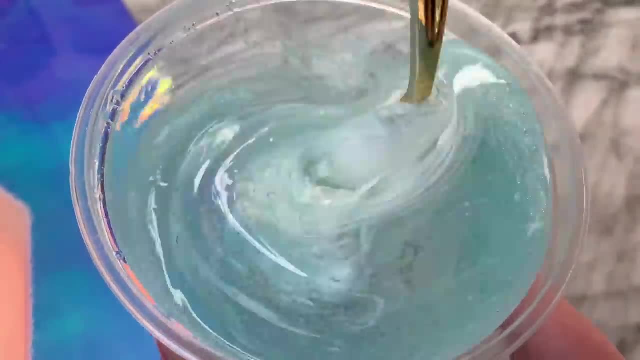 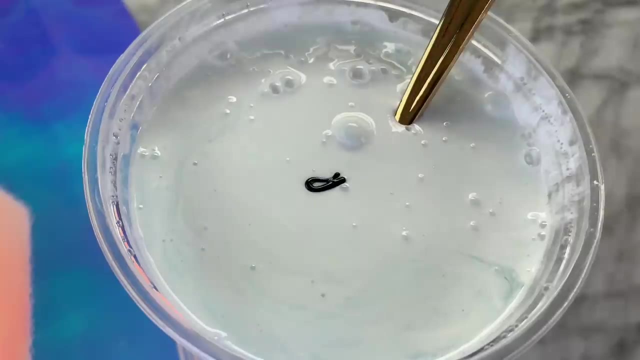 paint that i found in my house and then, once you add the acrylic paint in, you just want to mix all the ingredients together. at this point your ingredients should start thickening up because of the shampoo and dish soap combination. we have reached the fun part. we are going to dye our slime. 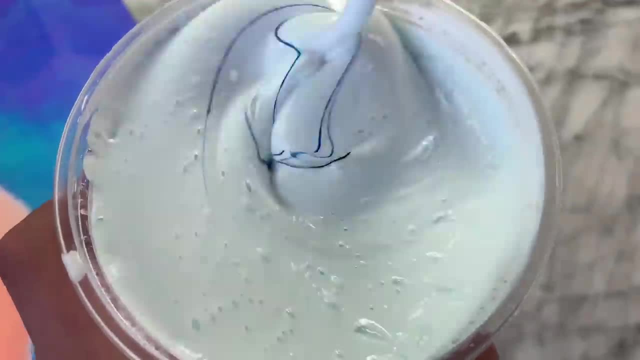 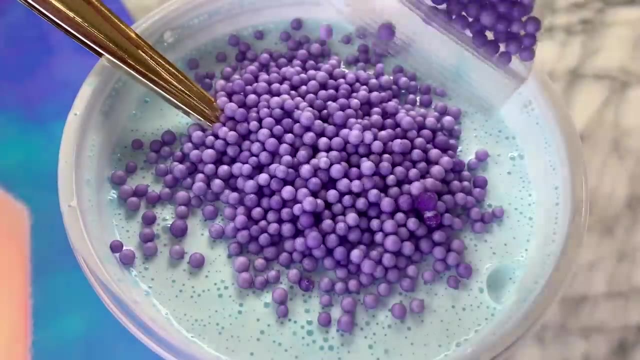 and color it and make it look really cool. so i'm going to be making mine a blue slime by adding in some turquoise blue food coloring, and i'm also going to be adding in some purple flowing beads. so i'm going to be adding in some purple blue food coloring and i'm also going to be adding in 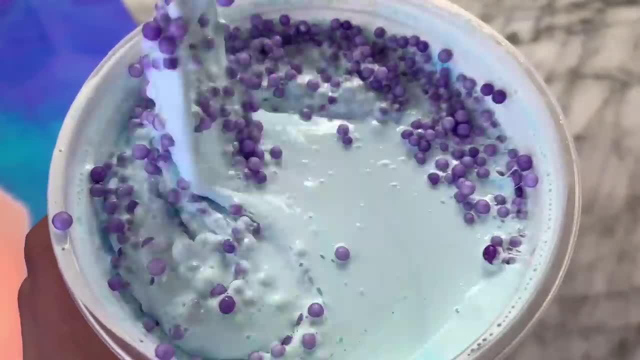 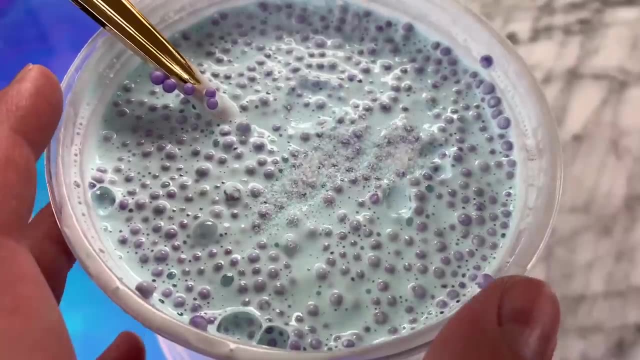 some turquoise blue food coloring and i'm also going to be adding in some purple blue food coloring to activate this slime. i will be using iodized salt. the difference between normal salt and iodized salt is that iodized salt has a element called iodine added to it and iodine salt just basically. 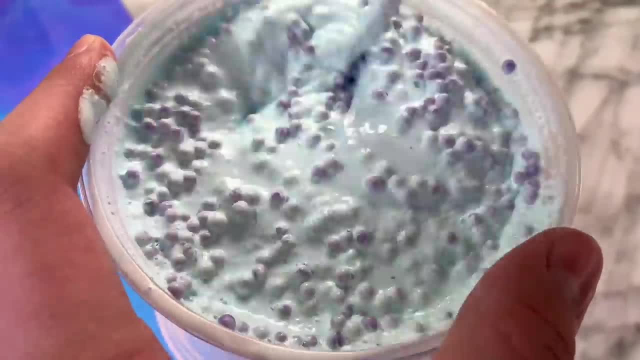 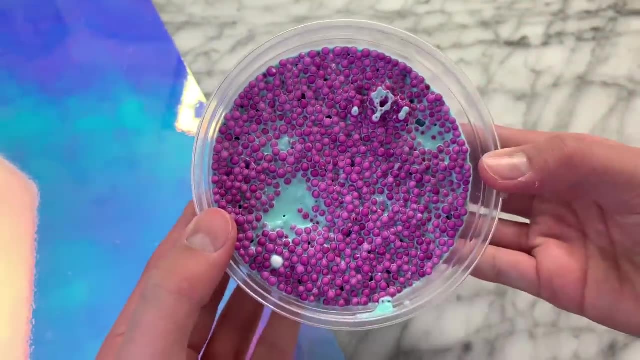 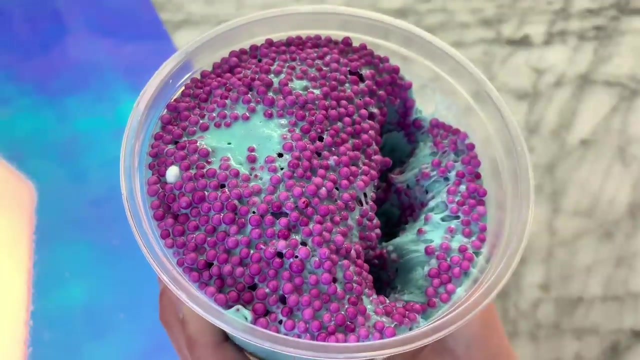 dries everything out better. so when you add it into the slime and let it sit for a little bit, the soap will dry out a lot more. here was the slime after i let it sit for a couple hours to dry out oil barely checked. so we are going to be adding some of the ionizing liquid to 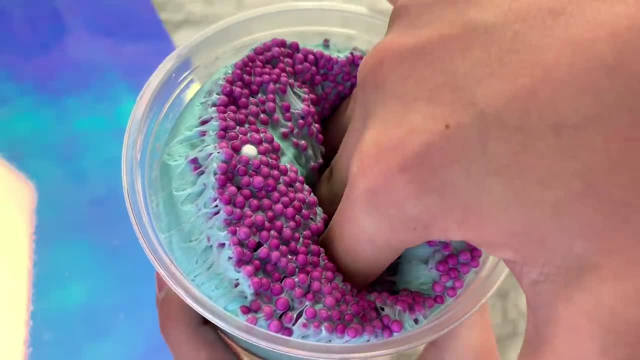 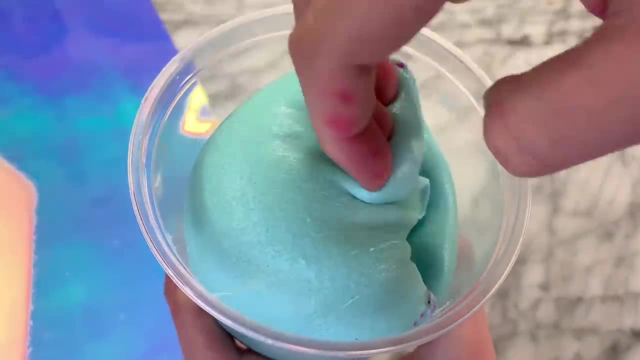 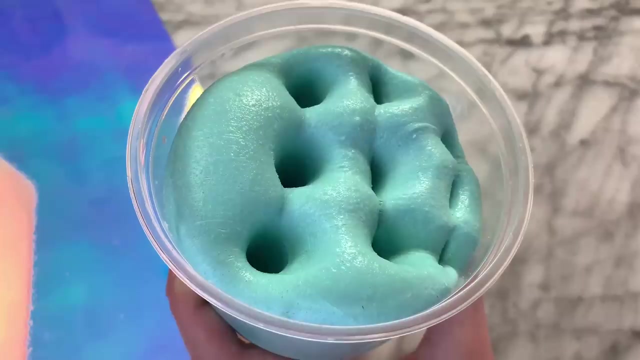 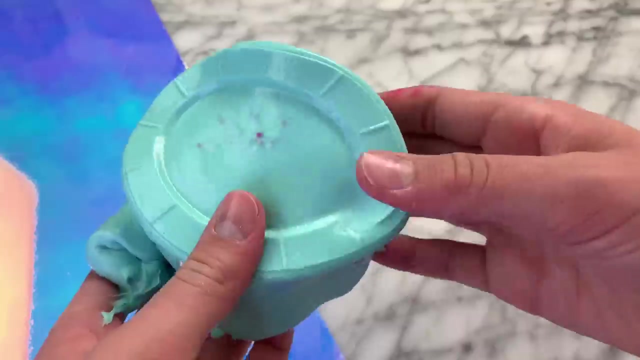 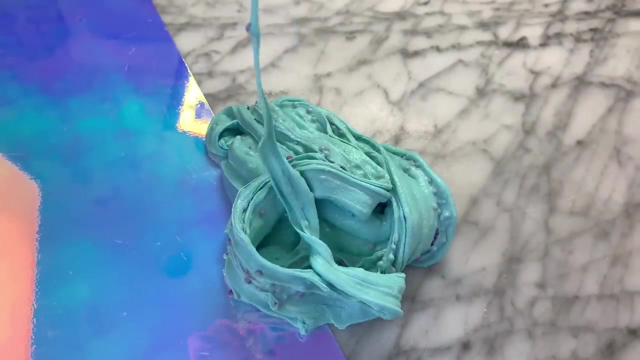 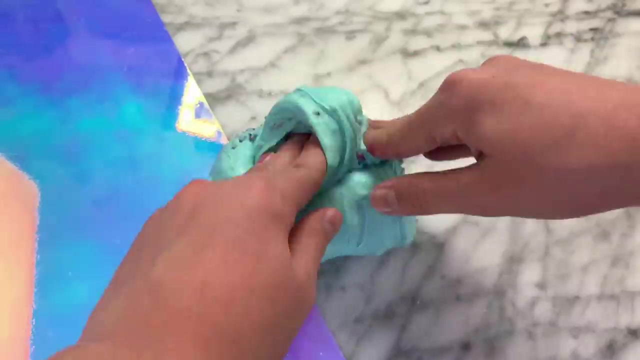 the isolated place to keep the drops from попадating to the incluso si yo, sino, si si ii, side to side like this. so so, so, so so. slime test will be super fun, because i'm going to be trying to make slime out of bubble gum. 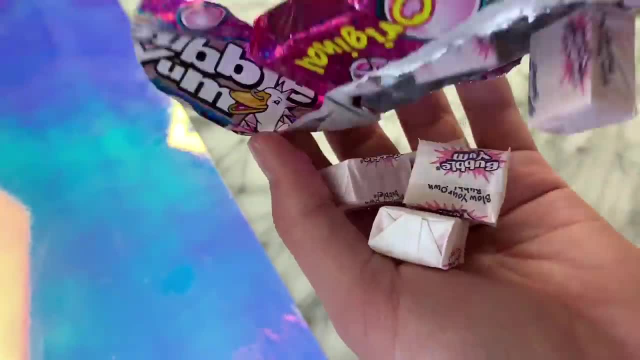 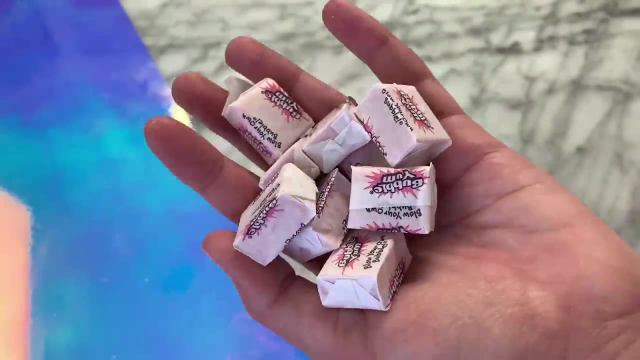 come up with a little plan to make bubble gum water slime. so what we're going to do is take some bubble gum, melt it in the microwave with some water, and then we're going to add some corn syrup to it and see if it will turn into a nice stretchy butter slime melting three bubble gums. 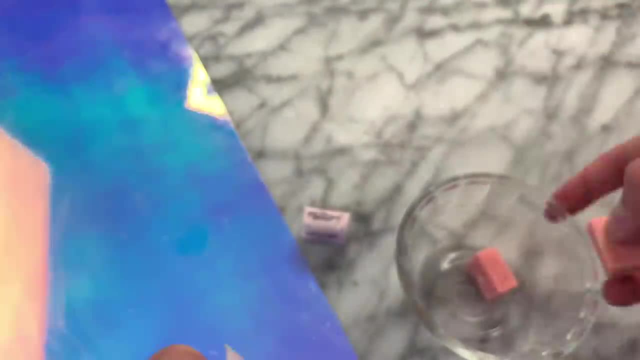 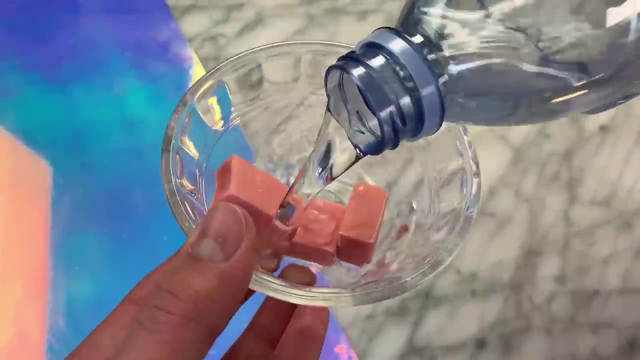 so that we can have a decent size slime now, just taking the wrappers off so i can pop them in the microwave and get them melted. now that i have my bubble gum in my bowl, i'm just going to add a little bit of water. i'm just going to melt this in the microwave. guys, i just took it out of the. 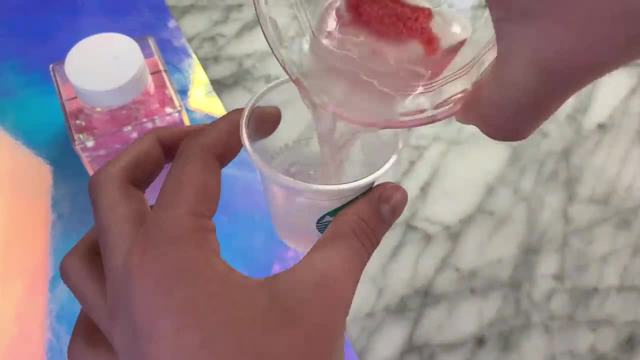 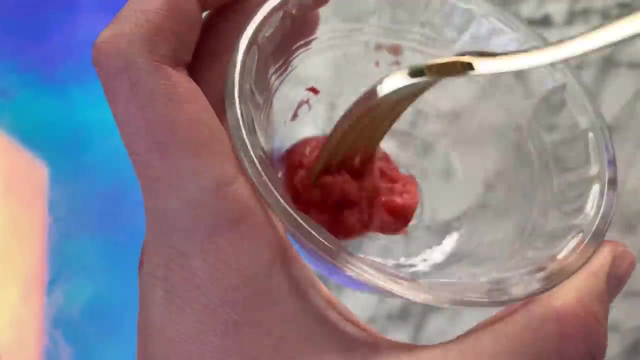 microwave and i'm just going to get rid of the excess water by putting in this separate cup. here is what the bubble gum looked like after i melted it. as you guys can see, it is really stringy, which was actually surprising. you can see it's really stringy. 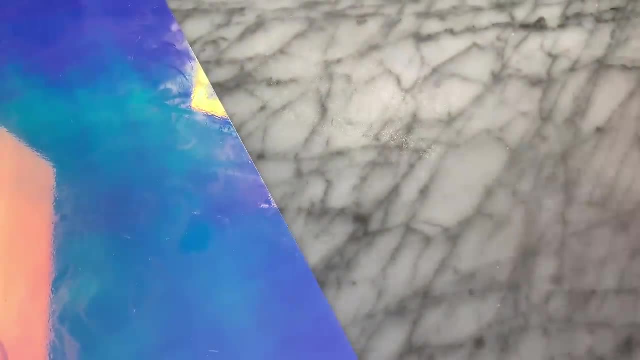 you can see it's really stringy, kind of looks like a cloud slime, but i'm just going to mix it up and then i'm going to add a little bit of corn syrup so we can make it less sticky and we can hopefully turn into a slime. 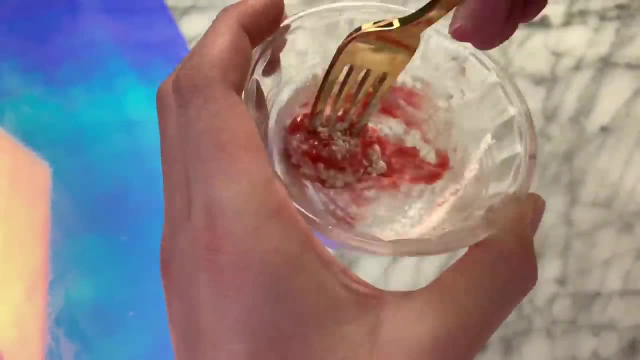 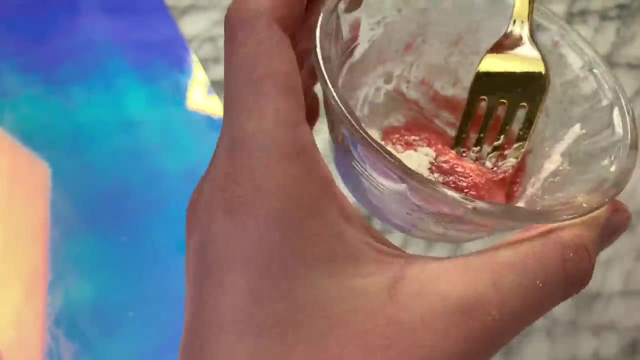 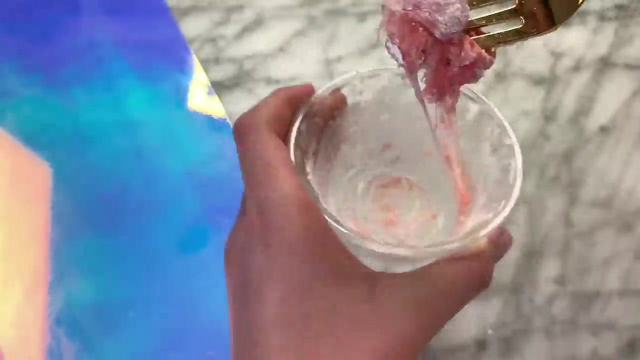 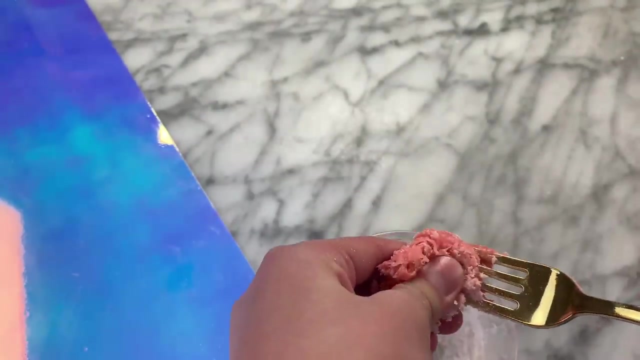 added a little bit of the corn syrup in, so i'm just going to mix it all together and we will see what happens. i'm kind of disappointed because it didn't get much less sticky and, as you guys can see, it wasn't slime like. so this slime was actually a fail. i'm able to get it dry, except for it just didn't stretch, so leave. 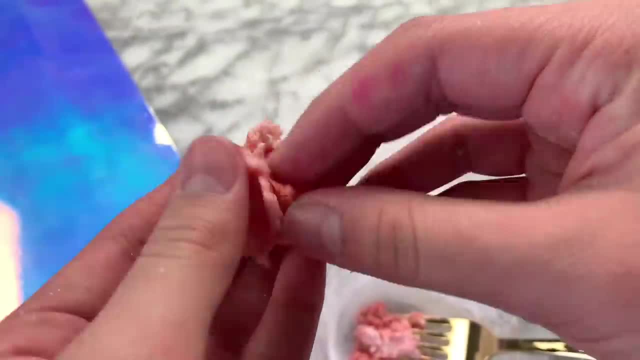 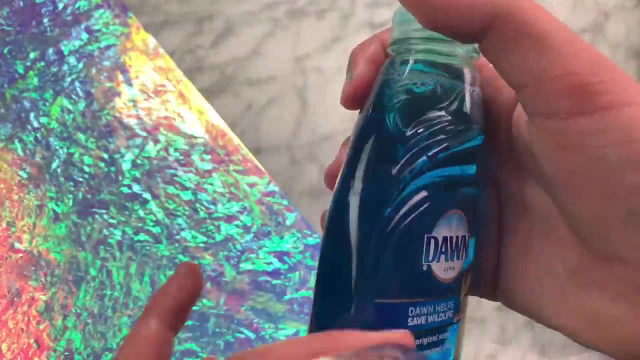 some recommendations in the comment below and try to find some more bubble gum recipes so i can test them again. i'm excited to show you guys the next time recipe because i will be showing you guys how you can make clear slime without any glue and out of just two ingredients: dish soap and listerine. so 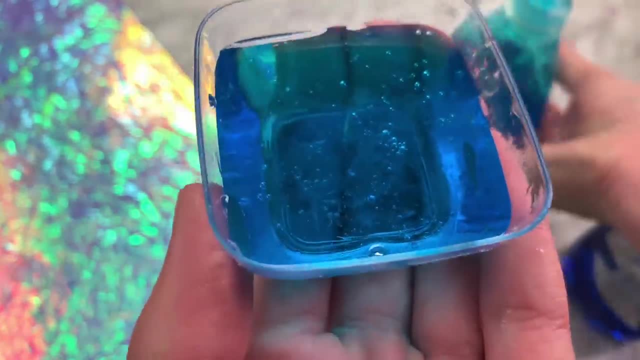 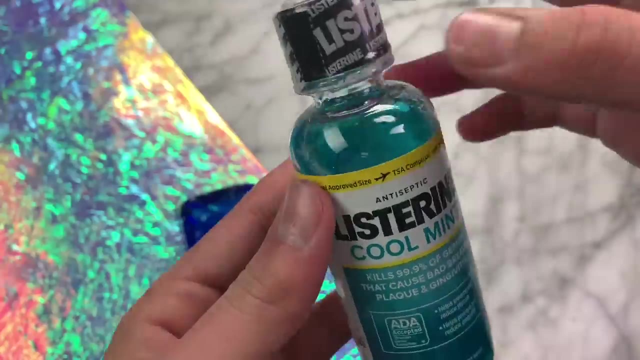 the first thing you need to do is just take some of your dawn dish soap- or whatever dish soap you're using- and just add it into two microwavable containers. basically, we're going to be using the listerine to help dry out the dish soap, and then we're going to microwave them and then we're 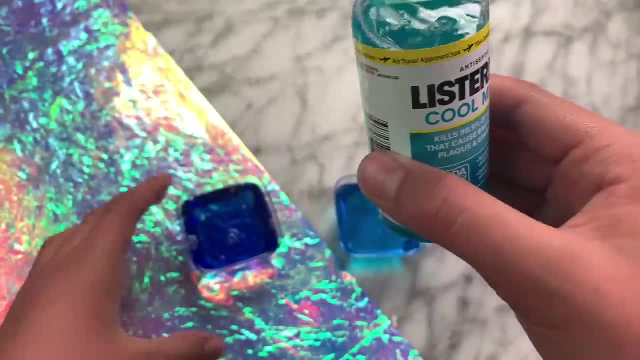 going to heat them up in the microwave so that we can turn them into more liquid form, so we can make them super dry and hopefully they will have a slime texture. any listerine will work for this. you just want to add a really small amount, because if you add too much it will won't work, so just add a. 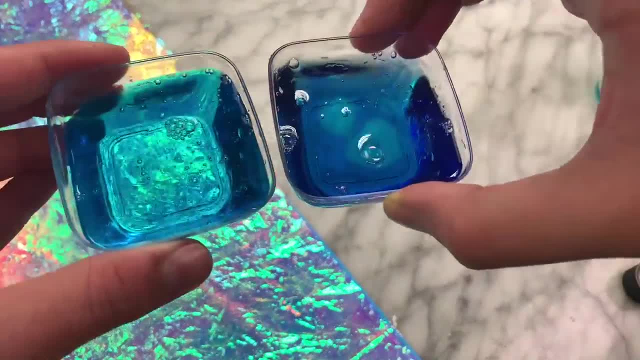 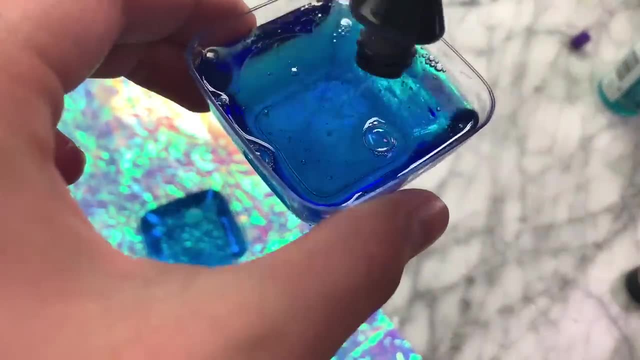 really small drop of listerine into each one of your bowls, or if you're just making one, just add it into your bowl of dish soap. i'm going to be adding a drop of purple food coloring into the purple one so i can make it a little bit more purple, because right now it's more blue and looks. 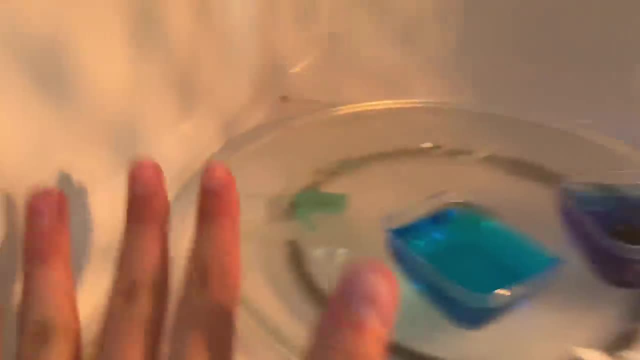 a lot like the blue one already. now we're going to just microwave them. it's really dirty right now. i need to clean it off. this microwave is dirty, so i will be using a small amount of listerine, which is the amount of listerine i will be using. 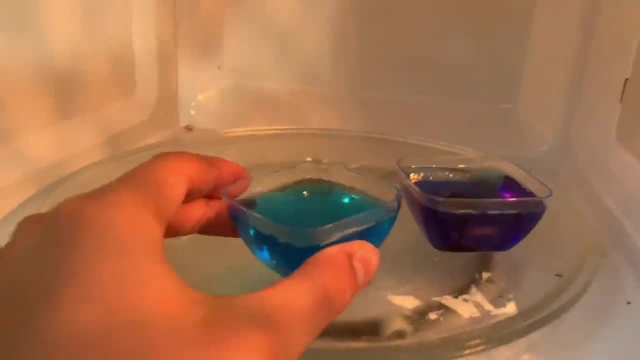 the microwave and i will be using the microwave because with this microwave, microwave is only used for slime, so it's super dirty right now, but I've just popped all- whoops. I've popped the two slimes in the microwave and we're going to just microwave. 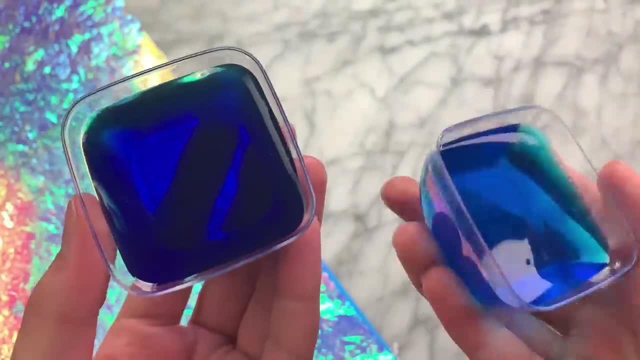 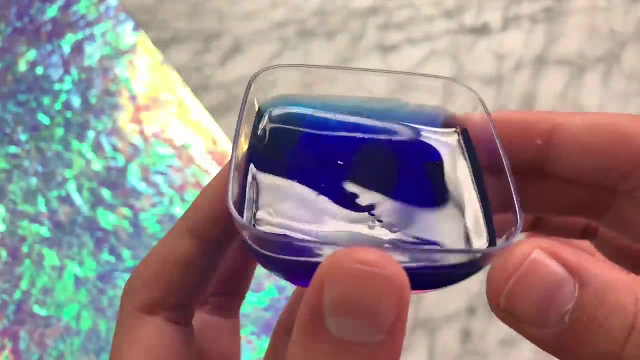 it for 30 seconds. Here's what our slime looks like. you can see they don't look super purple and blue, but in a second I will show you what it looks like when I put it by the window where there's lots of natural lighting. As you guys can see, they're not super sticky. 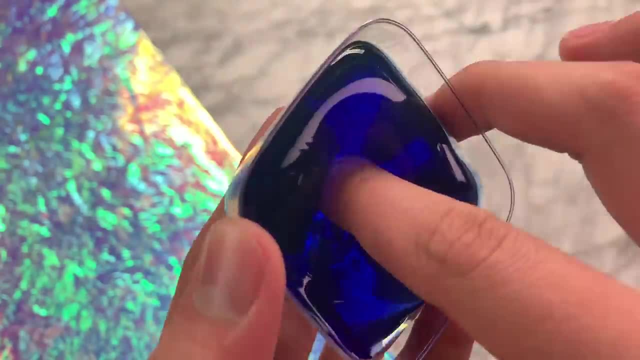 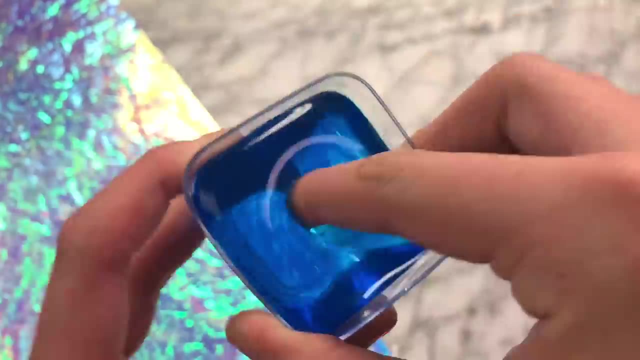 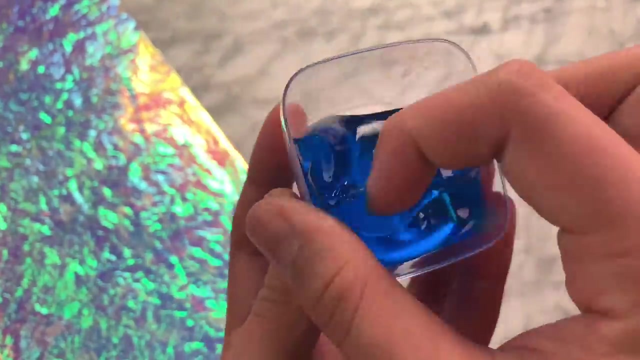 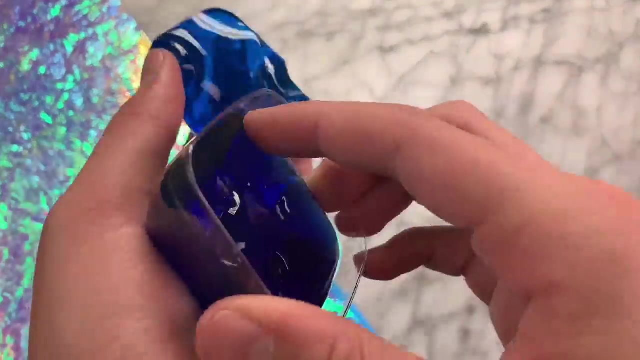 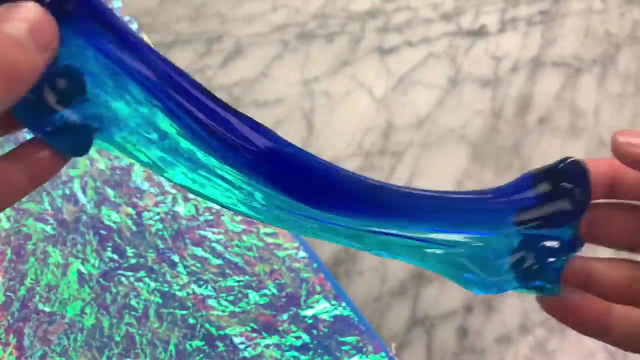 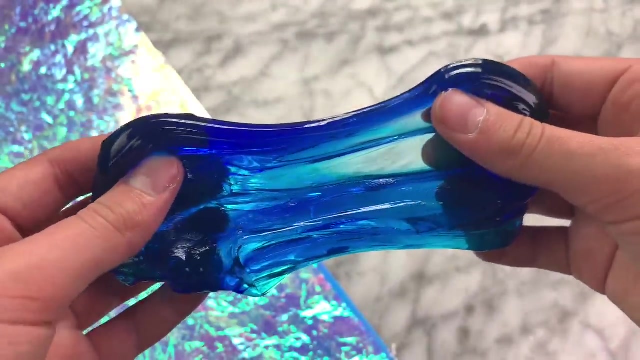 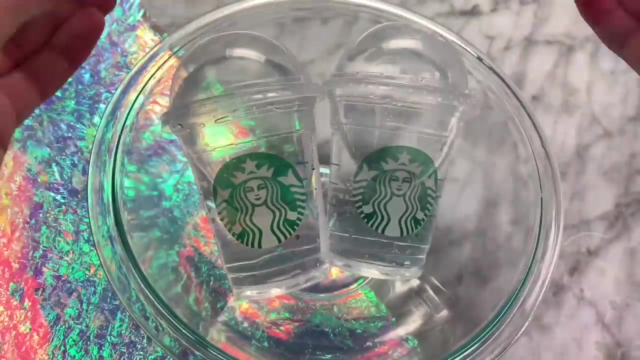 for being no-glue slimes, and they turned out just like slime Videos on Instagram that are super popular, where people will take two different colors of water and they'll add it into fake snow, so I thought it would be super fun to recreate. 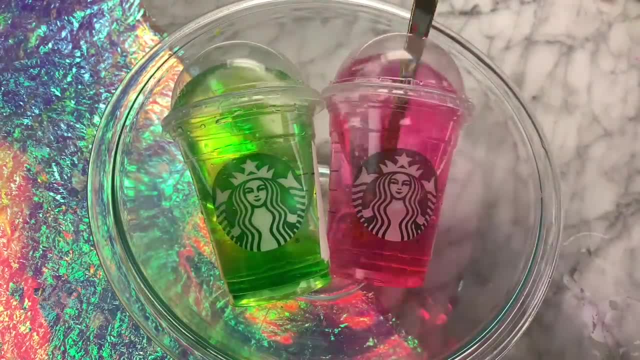 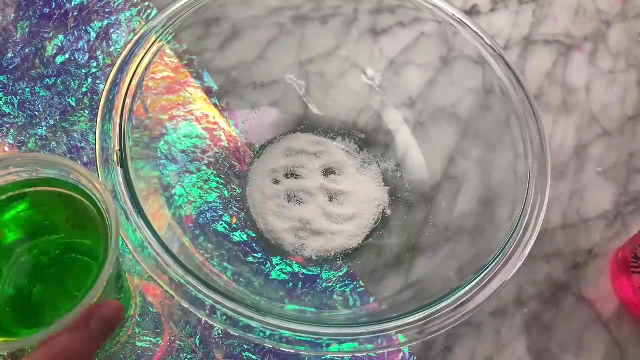 so I took these two empty Starbucks cups, just added some water and I added some colored food coloring and then I took some instant snow, I put it in my bowl and then I tried to pour the water in, But it basically just instantly blended the two colors together and it looked brown.